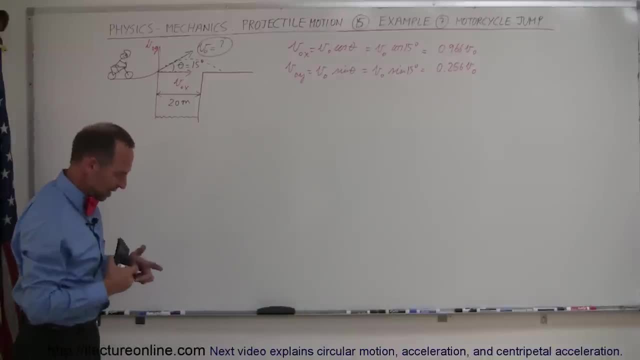 All right. So now we have our x and y components of our initial velocity, And by now you should guess that the next step would be to find the time in the air, Assuming that the takeoff point and the landing point are at the same height. let's just use that for simplicity. 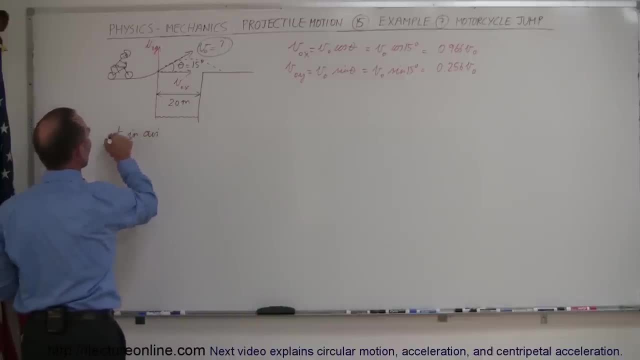 We can say that the time in the air can be found by using the equation: y equals y sub naught plus v sub naught in the y direction times time plus 1 half g t squared. That should be a very familiar equation by now. 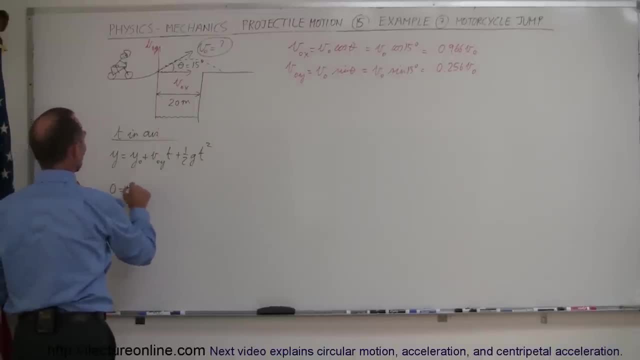 Initial and final height would be the same, So we can say 0 equals 0 plus initial velocity in the y direction That would be 0.256 v, initial minus 4.0.. I can't forget the time Got to have a time in there. 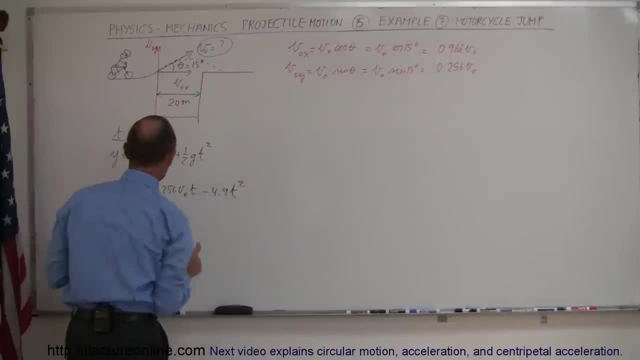 t minus 4.9 t squared. Now notice again: here we have the unknown v sub naught, which we're trying to find, And we have the unknown v sub naught. And we have the unknown v sub naught, unknown time. so we cannot solve for time with this equation wrong. but we can do. 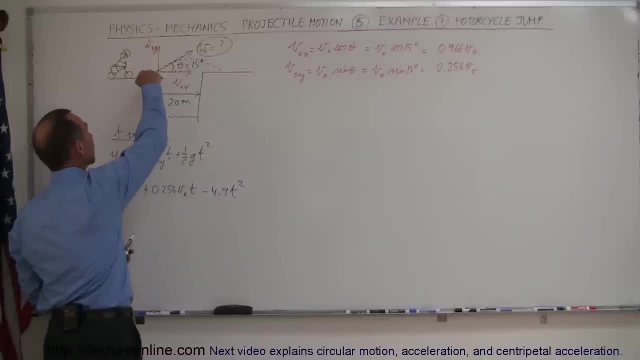 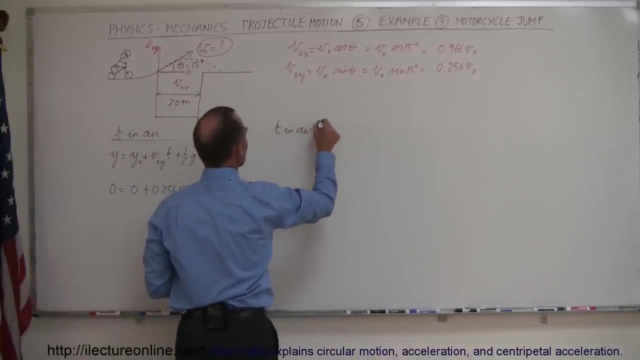 the same for the x-direction, because time in the air for the y-direction must be equal for time in the air for the x-direction. so let's do that. so time in the air using the x-direction equation. this was time in the air using the y-direction, so we have x equals V initial in the x-direction times time, or: 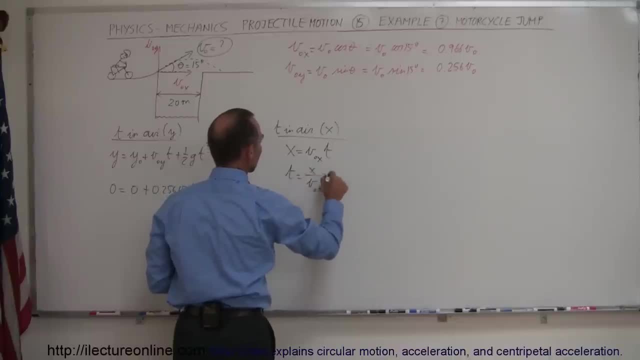 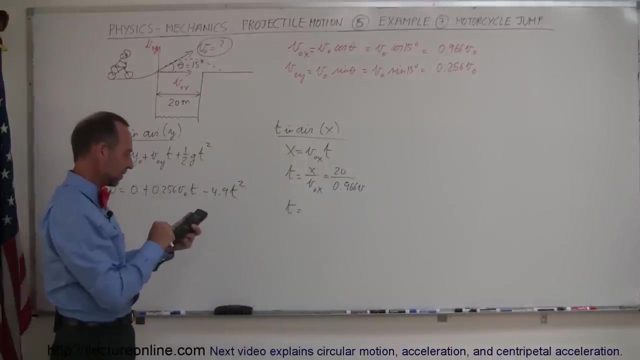 time is equal to x divided by V initial in the x-direction. in this case X is 20 meters, V initial in the x-direction is 0.966 V. so time is equal to: we have 20 divided by 0.966 equals, or 20.7 divided by V initial. I should call this V. 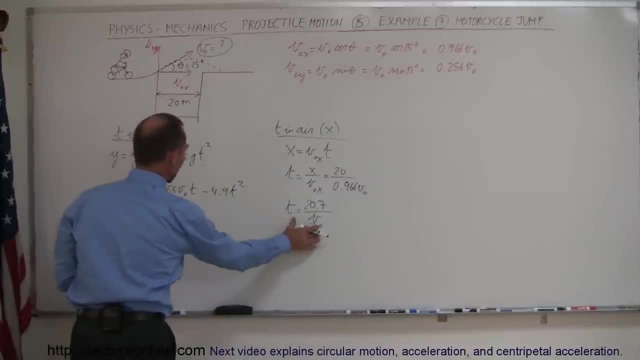 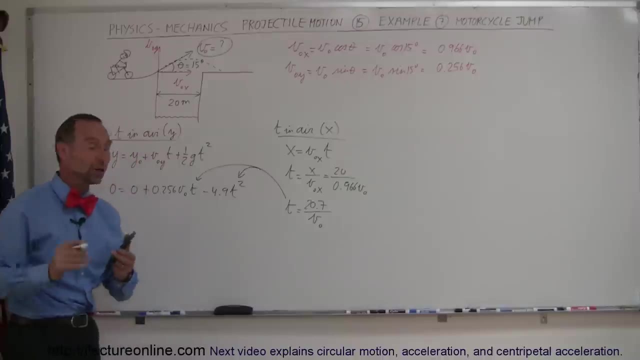 initial. all right. so now we have time in terms of V initial. here, here we have time and V initial in the same equation. we could then plug that in here and there and if we do that we only have one unknown left: V initial initial. all right, so we have 0 equals 0.256 V initial times 20.7, divided by V. 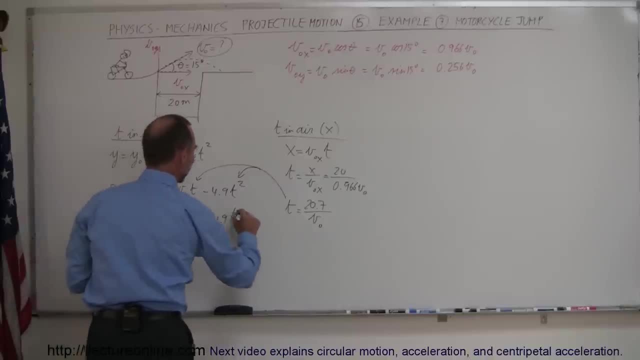 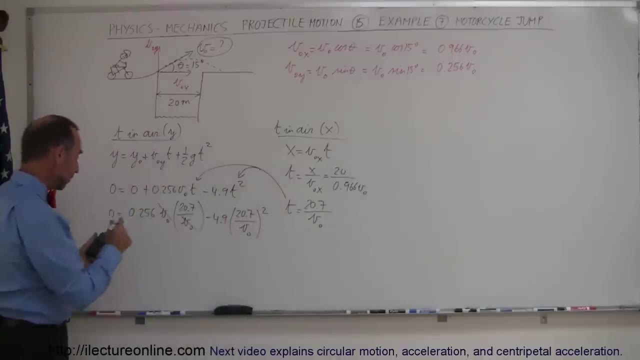 initial minus 4.9 times 20.7, divided by V initial quantity squared- notice, here the V initials cancel out- and simplifying this a little bit more, we get. 0 is equal to 0.256 times 20.7, so we get. 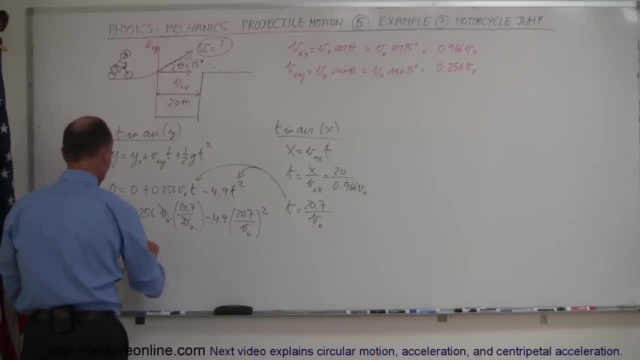 0 is equal to 1.966, so we get 5.3. is that correct? yep, so we have 5.3 minus. so we have 20.7 squared times 4.9. equals that would be minus 2100. so 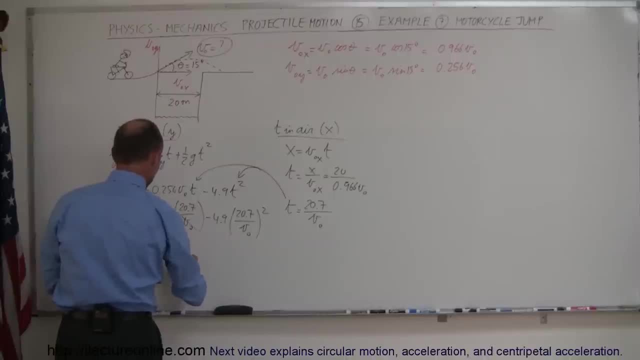 minus 2100 divided by V initial squared. ok, now you can see how this is simply solving for equation with V initial squared. so we're going to go ahead and move this over and turn the equation around, so we have minus 2100. so we have a very high equation here. looking for the equation with the equation withấ�係aves, Jordan's equation with kilos, this will 20102 divided by two- quarantine or more. so what we minus 2112 divided by V initials squared. and now you can see how this is simply solving for equation with padiplae to 2090 squared. so we're going to go ahead and move this over and turn the. Oh well, let's see here. 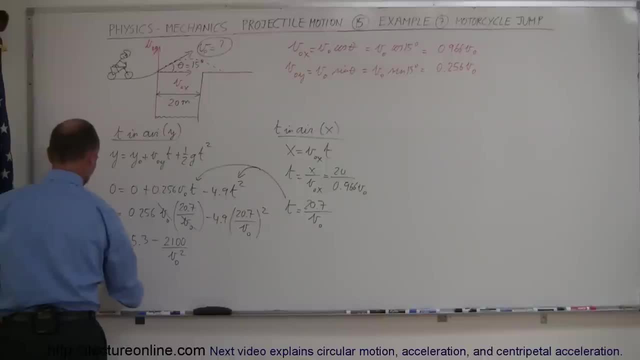 What's the best way of approaching it? Let's just move to minus 5.3.. So minus 5.3 equals minus 2,100 divided by- I'm missing a 1 there- 2,100 divided by V, initial squared. 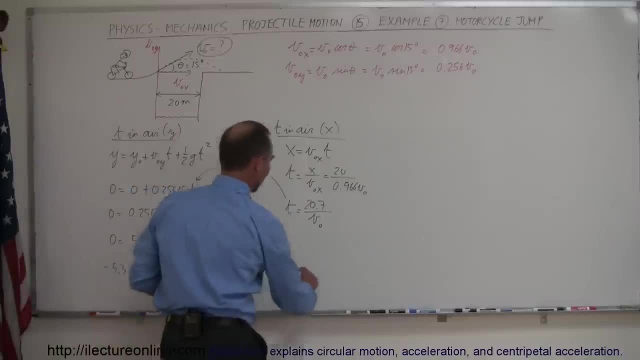 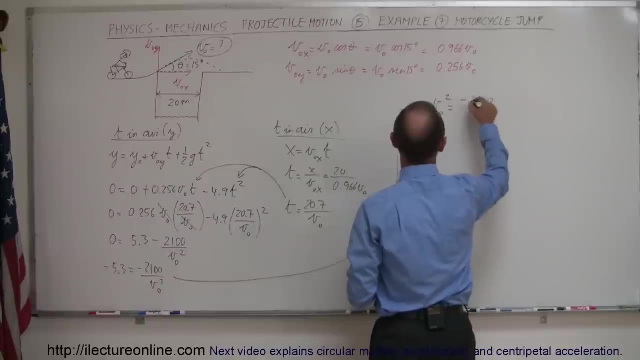 Moving this over here and this down there and moving this way so I have more room. So I have V. initial squared is equal to minus 2,100 divided by a minus 5.3.. Notice, of course. then the negatives cancel out. 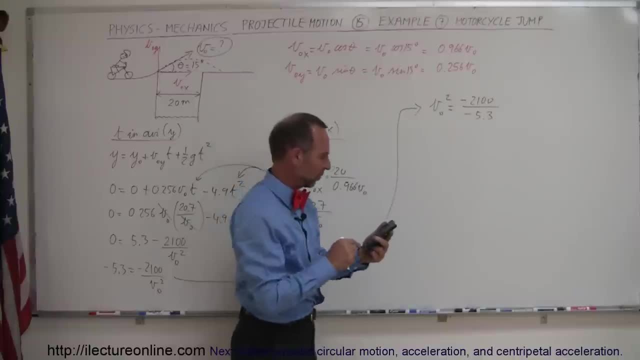 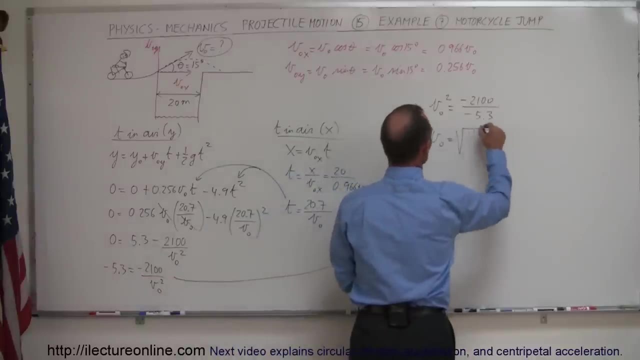 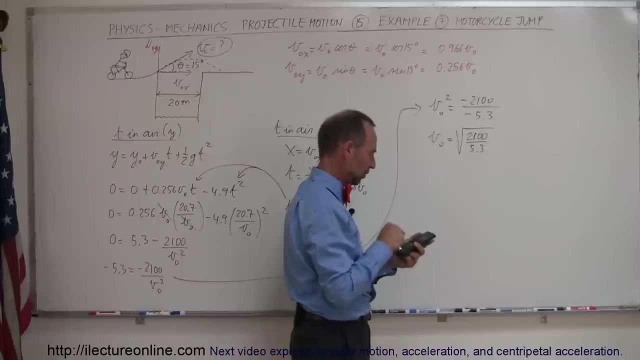 So we have this: divided by 5.3 equals. so we have V. initial is equal to. and then, of course, taking the square root of both sides, the square root of 2,100 divided by 5.3.. Take the square root and we get 19.9.. 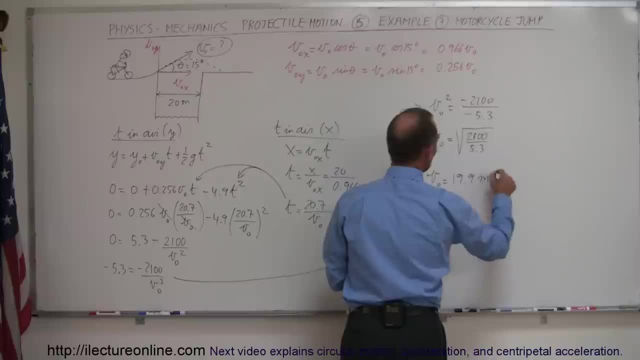 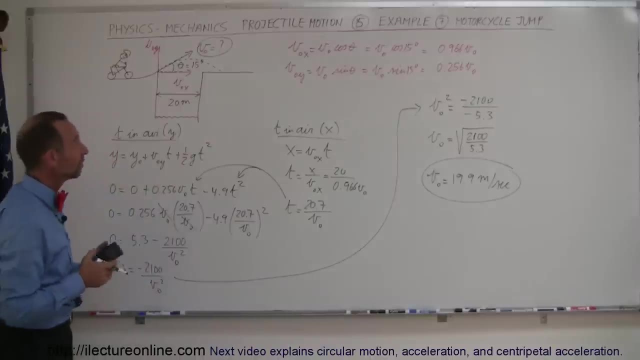 V initial equals 19.9.. Of course the units are meters per second. All right, so if Evel Knievel takes off at a speed of about 20 meters per second or faster, he'll make it across the canyon. Anything less than that, that might spell problems. 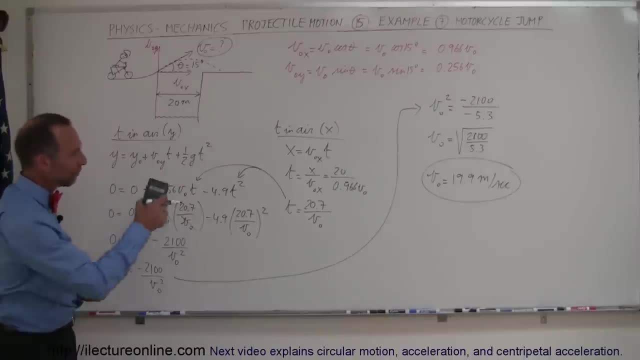 Of course, assuming there's some wind and friction and all that, I would go a little faster than that, just to make sure I'd make it across that canyon. Of course I wouldn't be that crazy to try that. All right, that's how you do that problem.